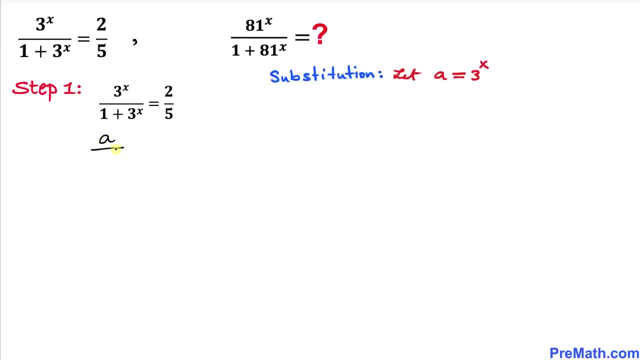 substitution could be written as: a divided by 1 plus a equals to 2 divided by 5. and now let's go ahead and cross multiply, so that is going to give us 5 a equals to 2 plus 2, a subtract 2: a from both. 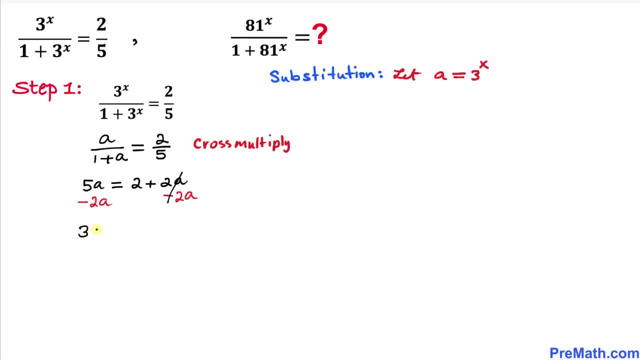 side. this is gone. so we got 3. a equals to 2, so that means our a value turns out to be 2 over 3, and here's our next step. let's focus on this expression: 81 power x divided by 1 plus 81 power. 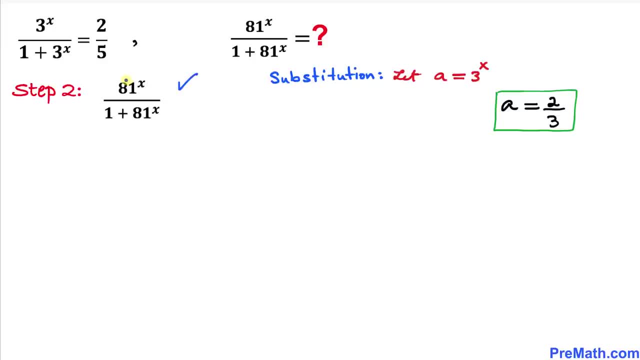 x- and here i have copied it down, and let's focus on this base 81, and here i have copied it down and let's focus on this base 81, and here i have copied it down and let's focus on this base 81. and 81 could be written as 3 power 4, so therefore we can write this expression as 3 power 4 whole. 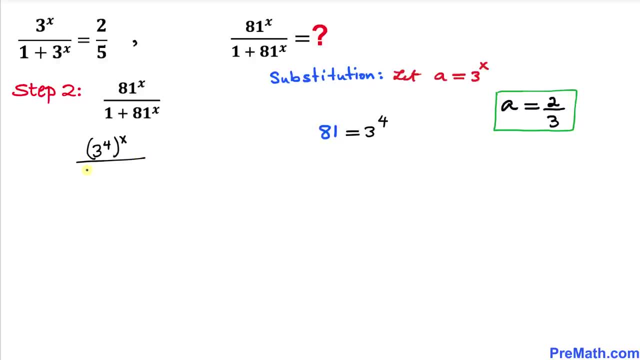 power x divided by 1 plus 3 power 4, whole power x. now let's recall this power rule of exponent: x power a, power b could be written as a, x power a times b, and likewise x power b, and then power a could be written as x power. 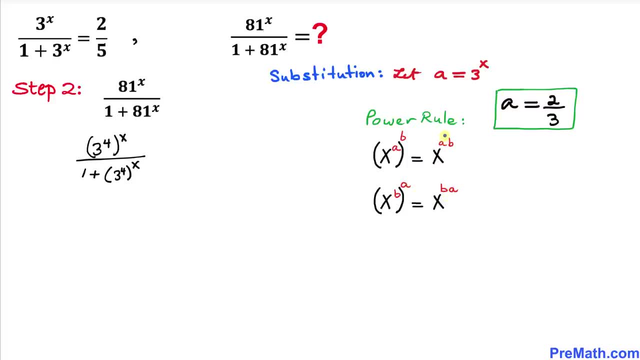 b times a, and now we can see that this exponent a times b is same as b times a. so therefore we can see that the right hand sides are same. if the right hand sides are same, then our these left hand side are going to be same as well. 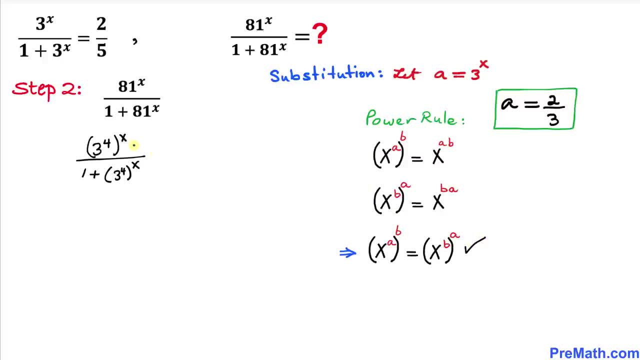 so therefore, we are going to apply this rule to this given problem over here, so this could be written as 3 power x and then power 4, divided by one plus likewise, 3 power x and then power 4, and 3 power x is same as b and then power 4. we know that our this three power x is the same.